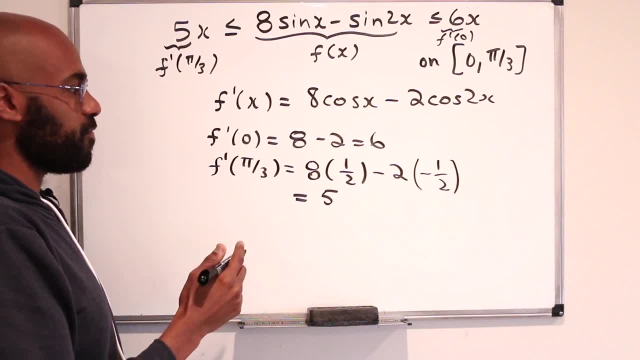 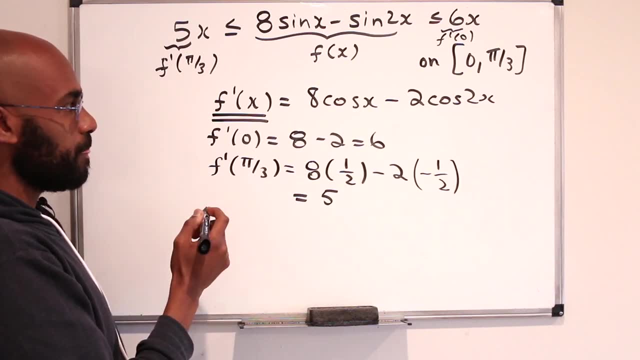 Now we could do something like that if we had some information about the nature of this function itself. Does it decrease, Does it increase? We can find that out by looking at the derivative of it, which is the second derivative of our original function. 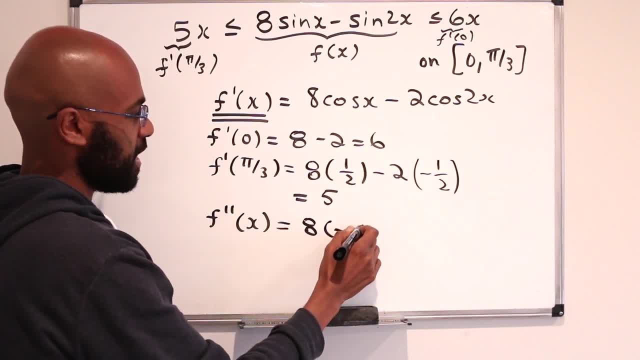 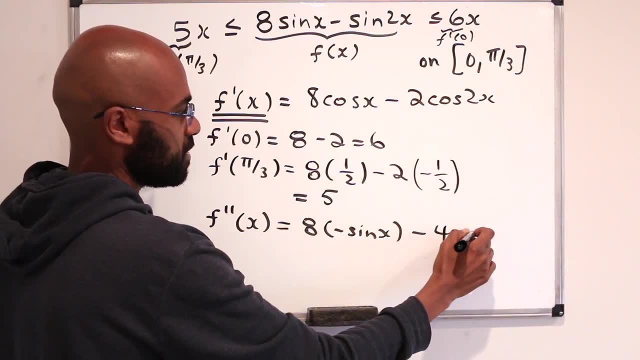 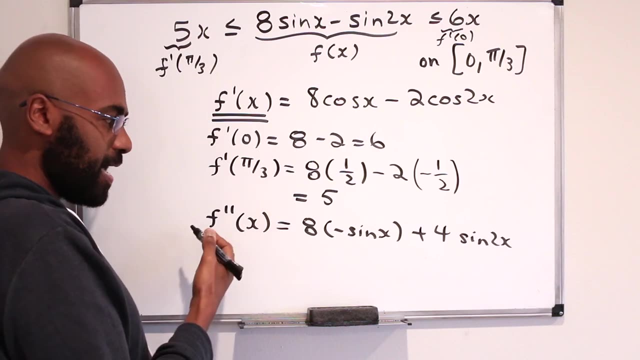 That would be 8 times negative sine x, Minus by a chain rule, again 4 sine 2x. But then we have a negative, so we get a plus here. Okay, to analyze whether or not the derivative is an increasing or decreasing function. 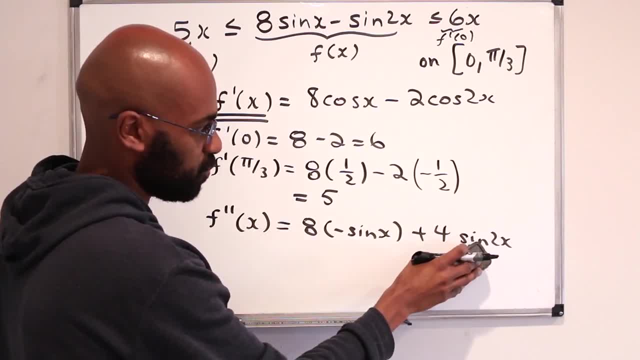 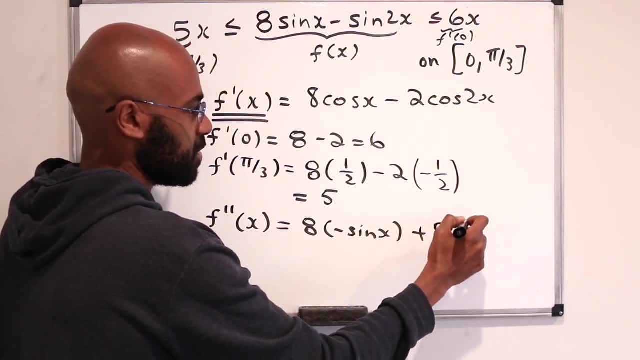 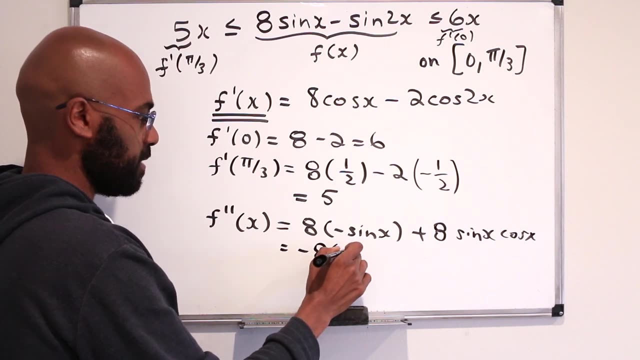 it would be nice to factor this. We can do that by changing this to a 2 sine x cosine x, So this 4 becomes an 8. So we get 8 sine x cosine x here, And so that gives us negative 8 times sine x as a common factor. 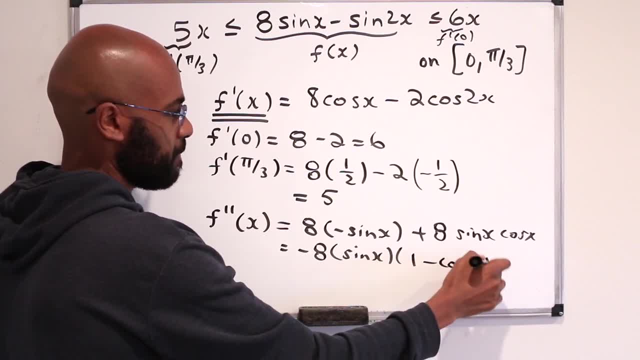 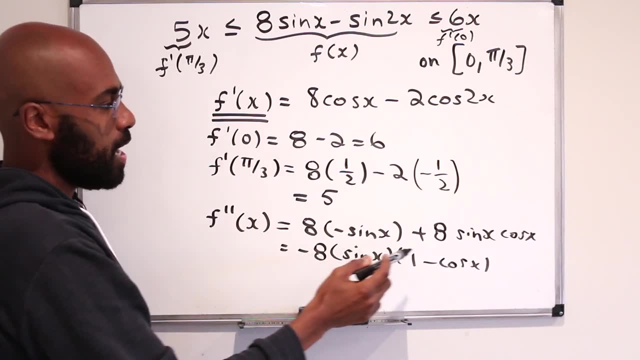 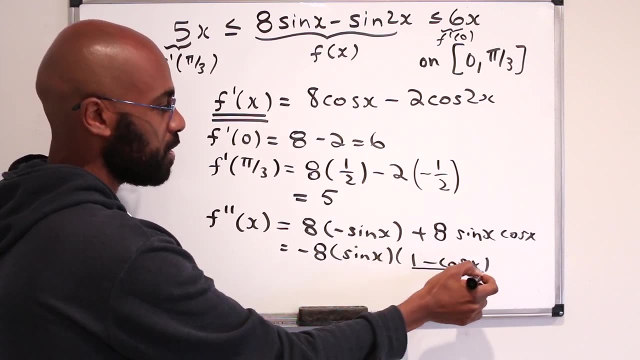 and then a 1 minus cosine x. All right, in this interval here, sine of x is non-negative And cosine x is non-negative as well, And since cosine x is bounded above by 1, this quantity here is going to be non-negative. 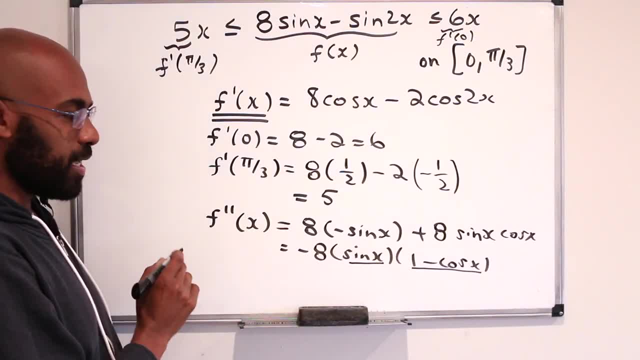 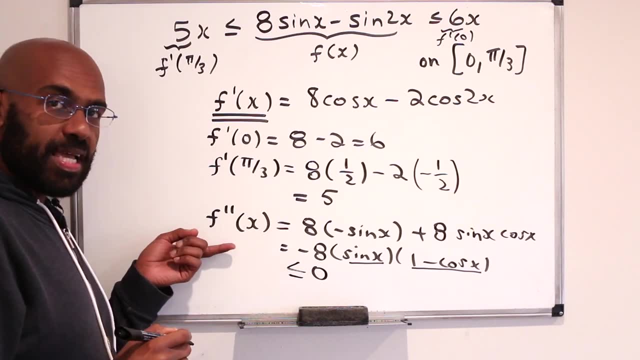 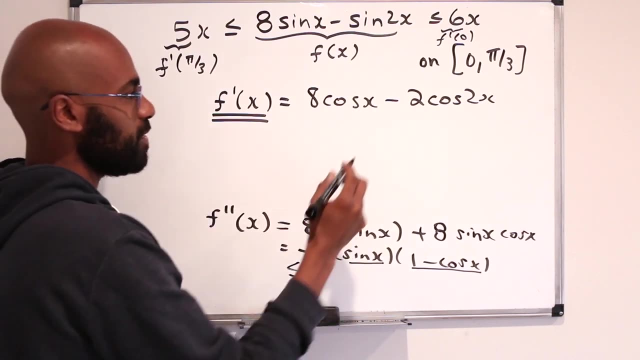 So we have a non-negative value. a non-negative value, and we'll multiply, That means the second derivative is less than or equal to 0.. So the second derivative is non-positive, which means the first derivative is weakly decreasing. Okay, so what this means then is if you pick any y in the interval 0 to pi over 3,. 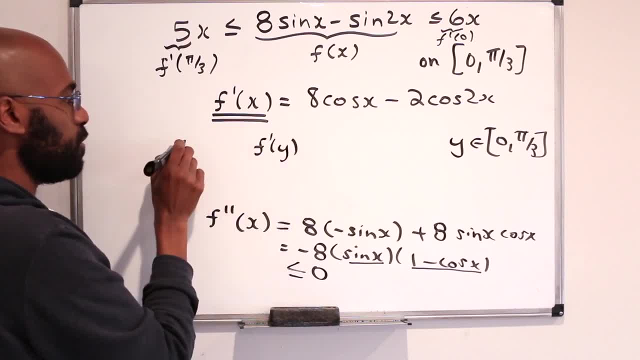 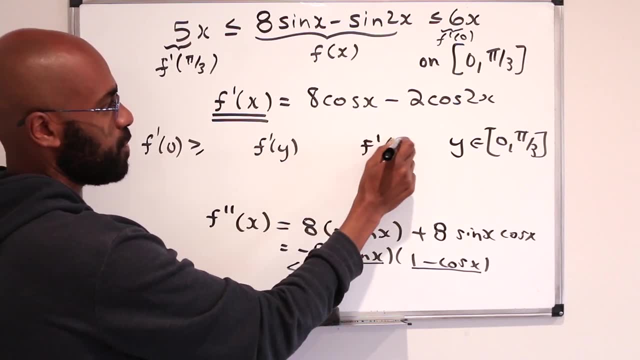 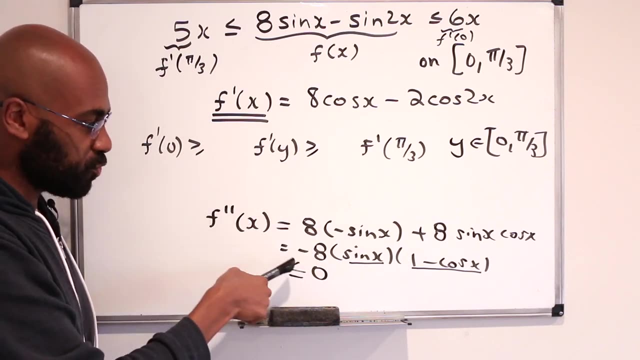 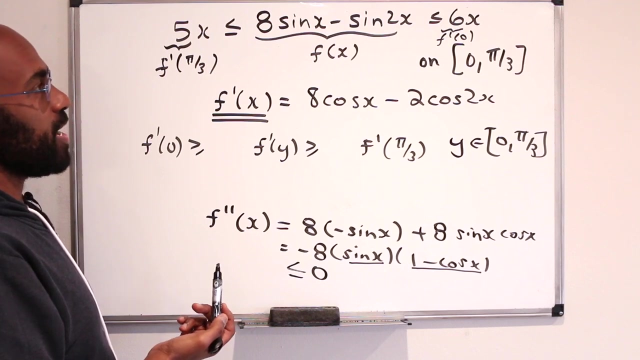 then f prime of y sits sandwiched in between f prime of 0 and f prime of pi over 3.. Because the second derivative, the derivative of this, is actually a non-positive number. Okay, great. So how can we use that to our advantage, figuring out a relationship between these values and f?